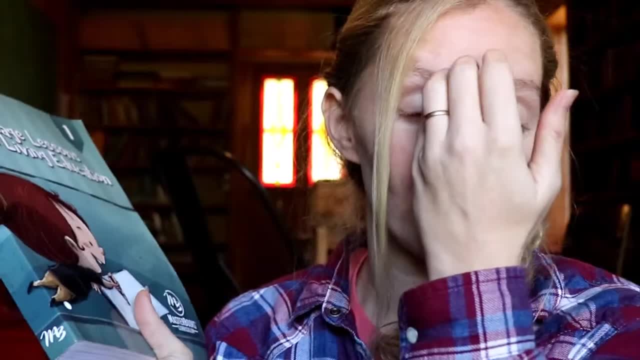 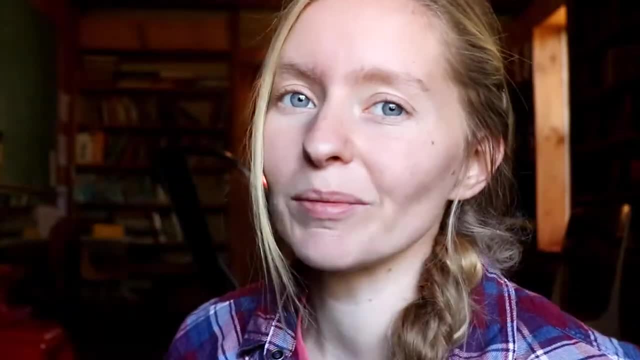 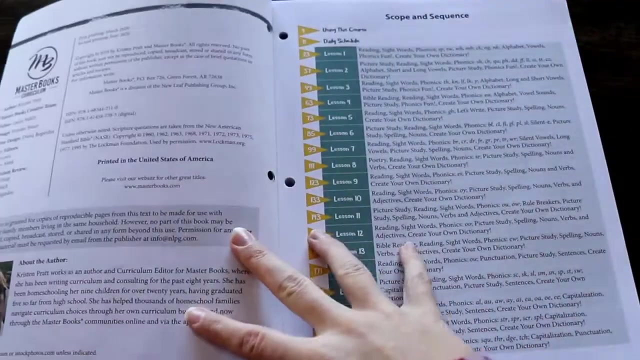 can do that easily. I just kept it in the book because it just seems easier to keep it in the book, But anyway, so let's get into the flip-through. So let's get started, So let's get started. 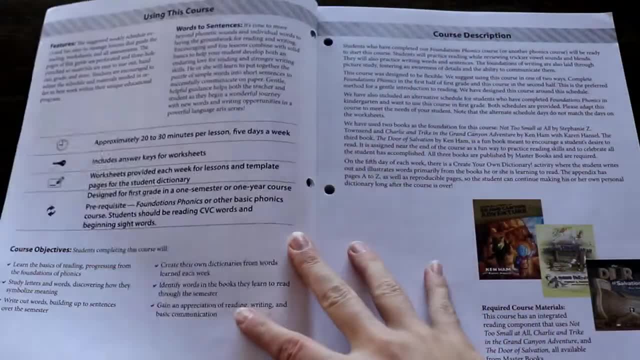 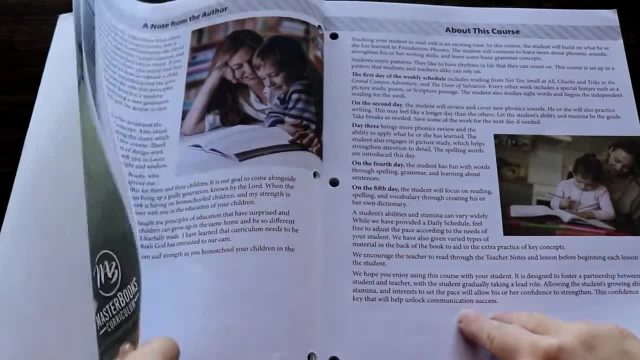 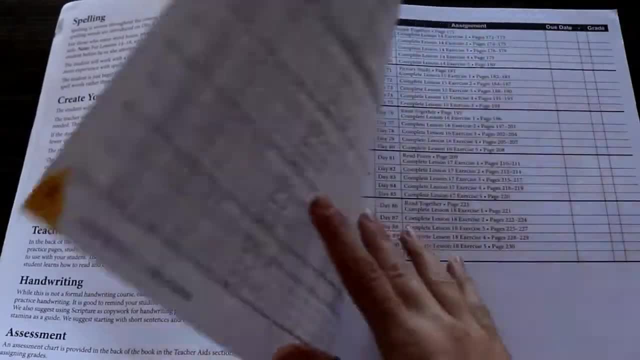 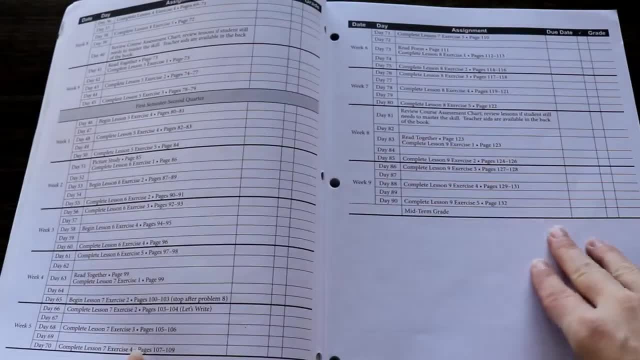 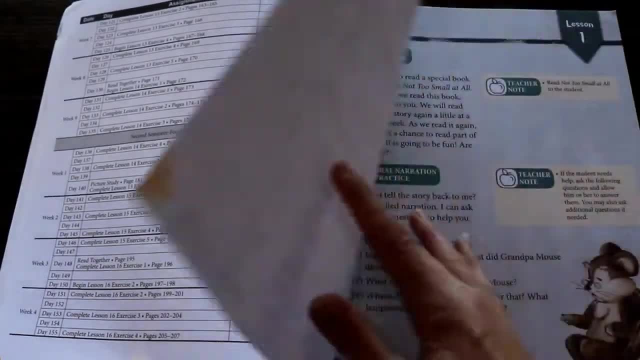 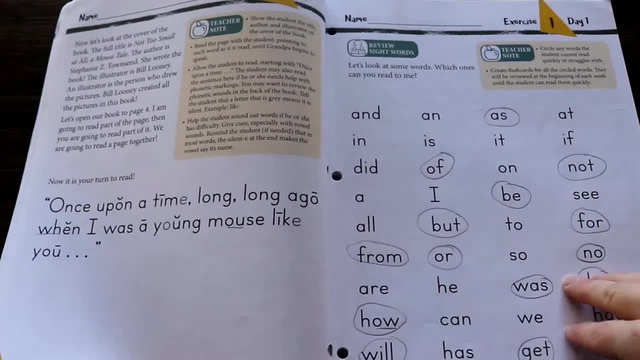 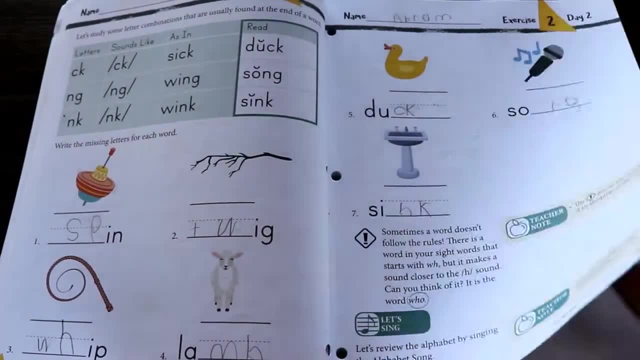 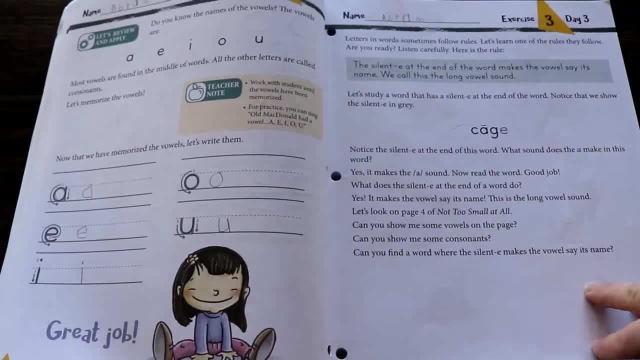 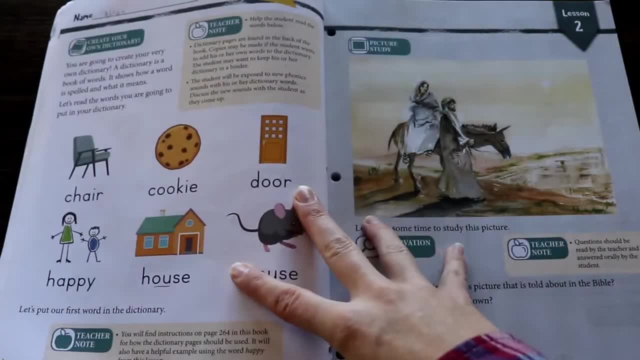 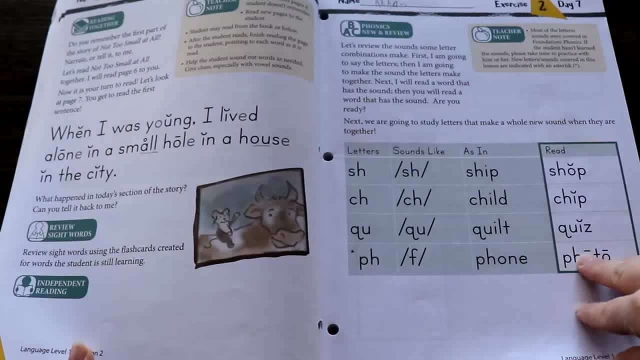 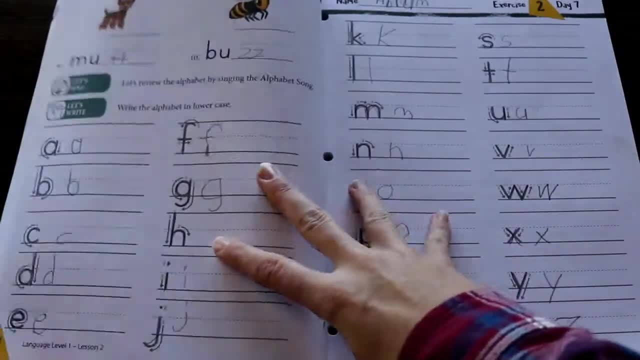 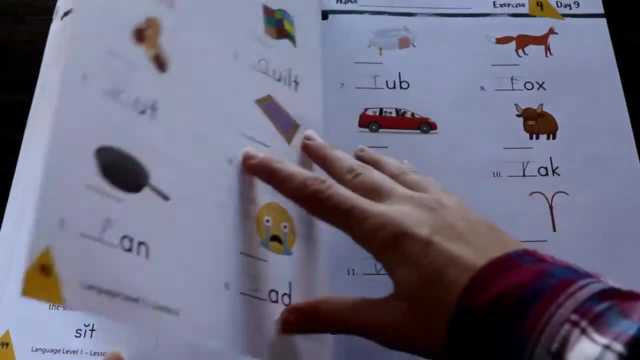 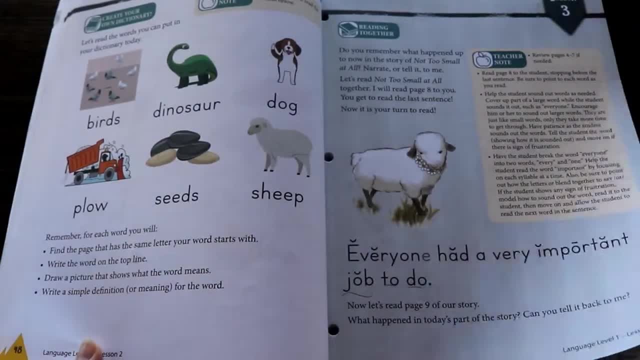 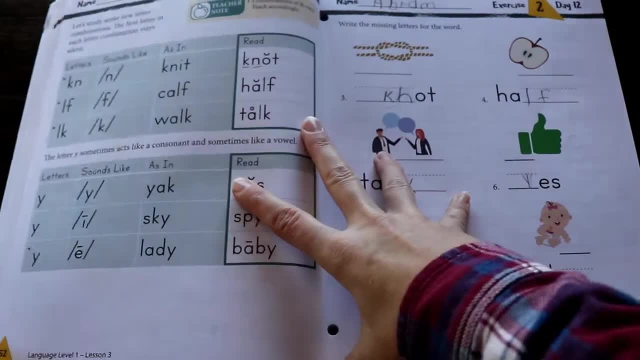 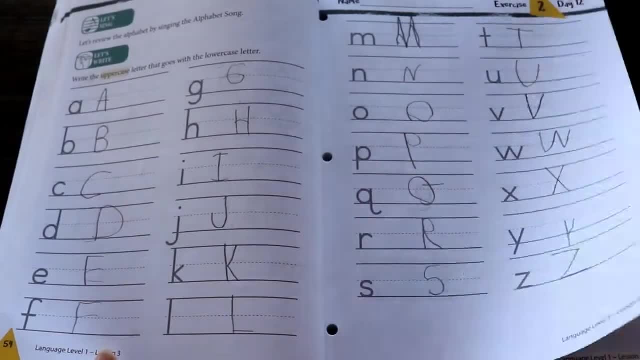 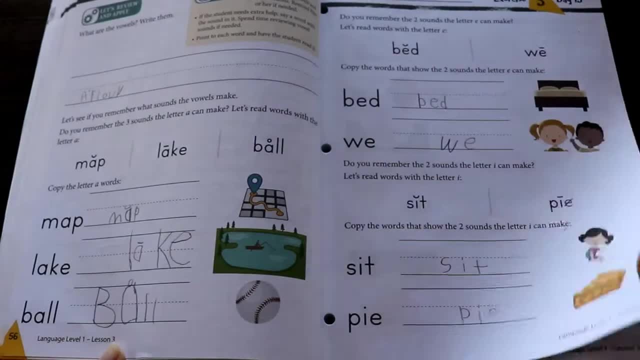 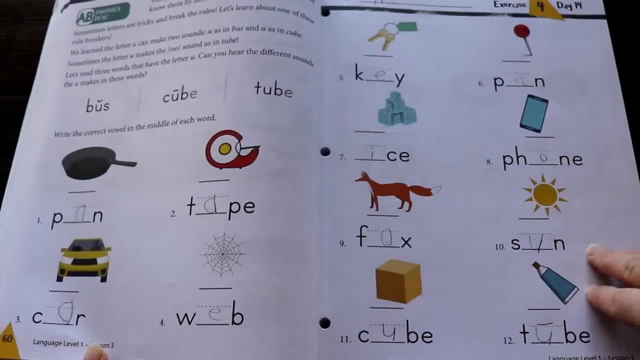 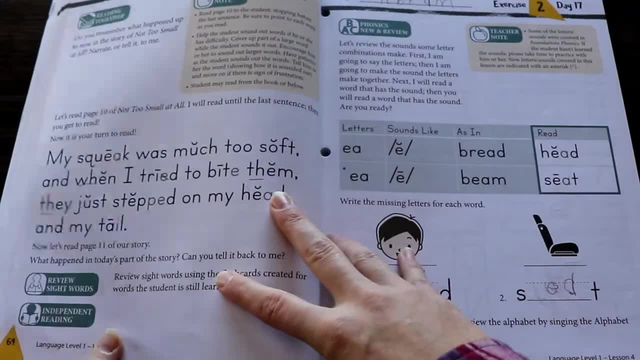 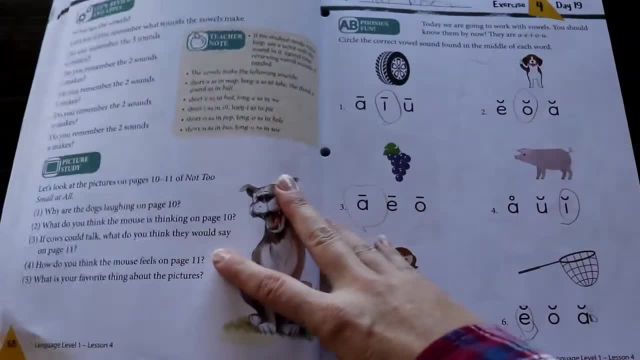 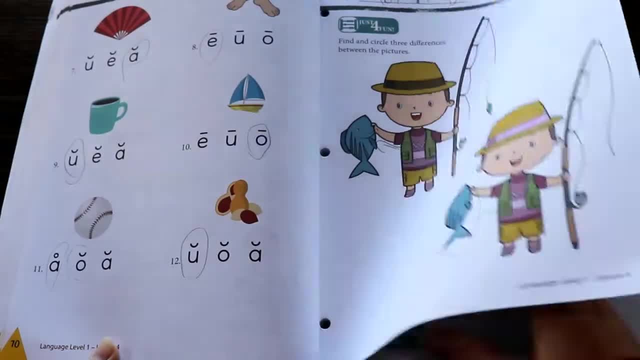 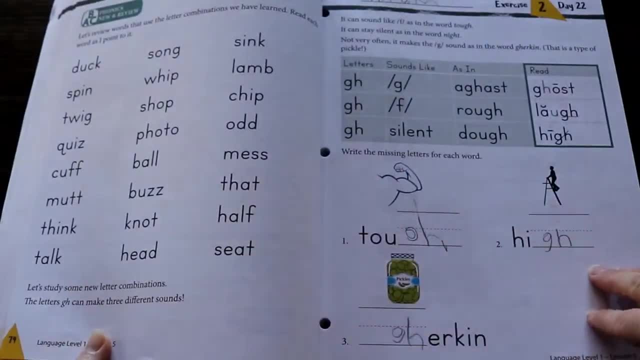 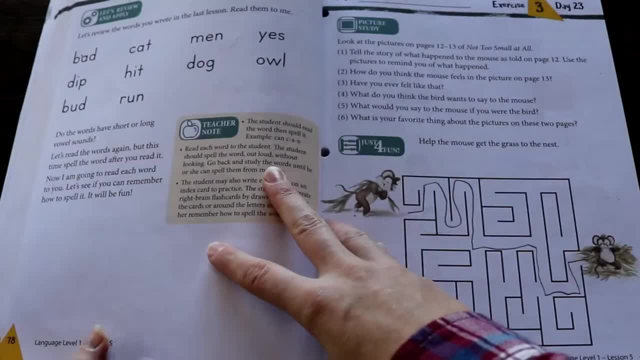 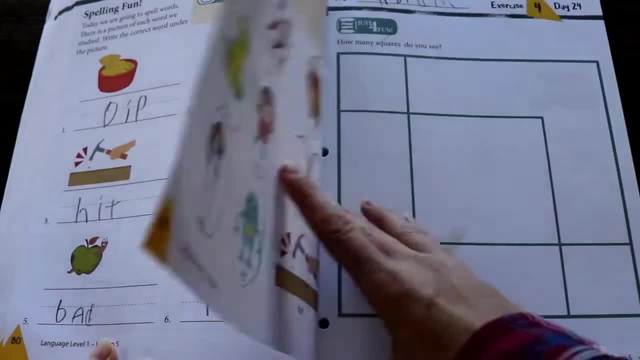 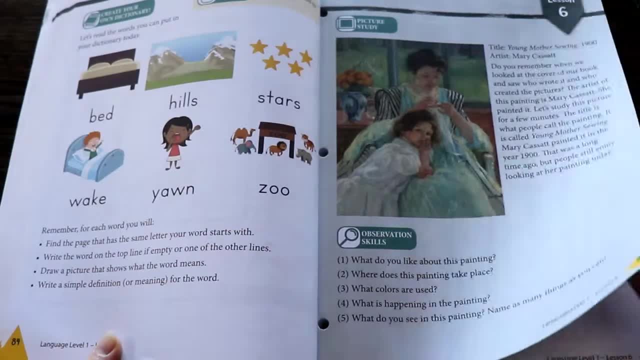 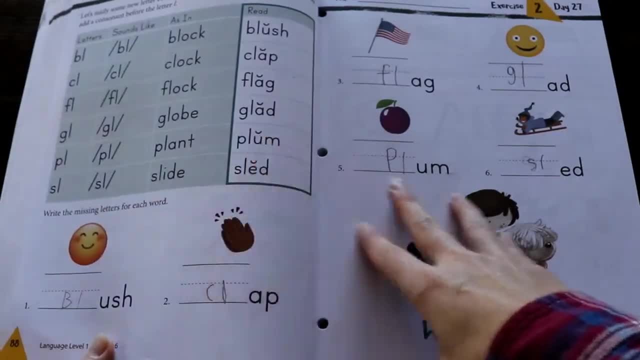 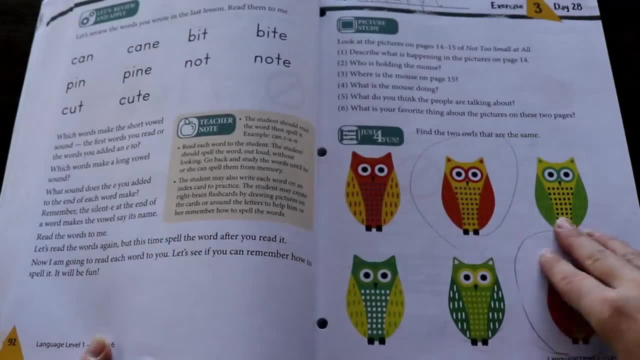 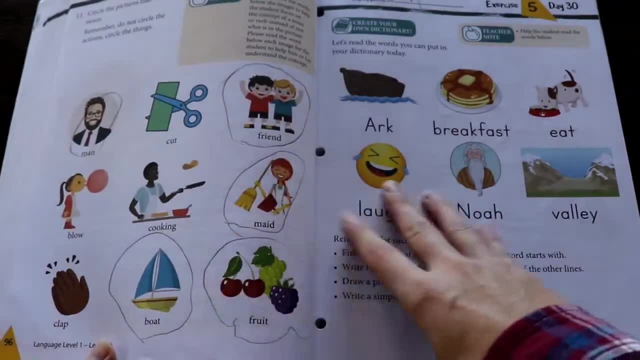 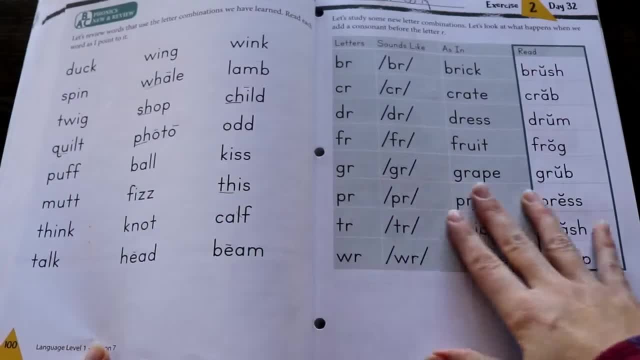 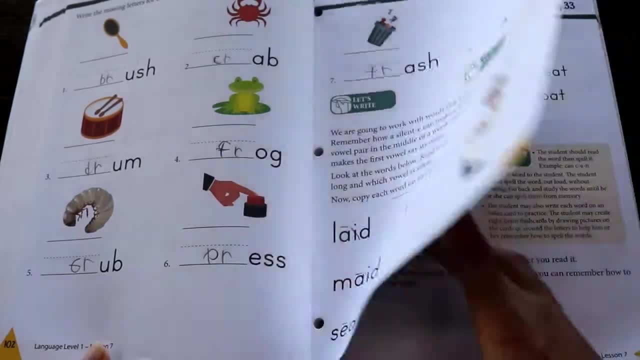 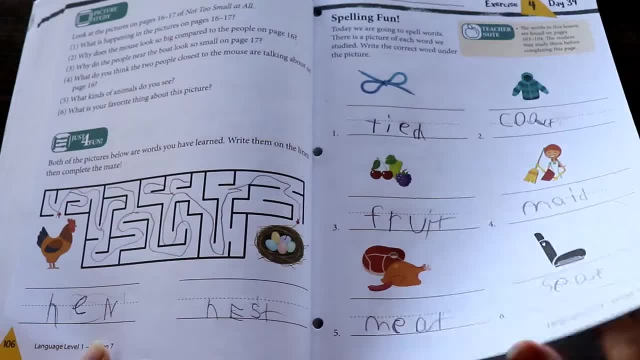 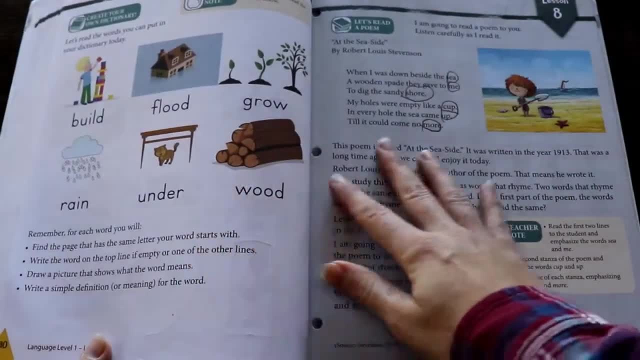 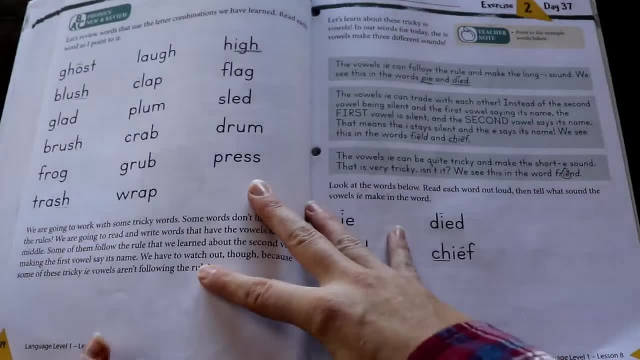 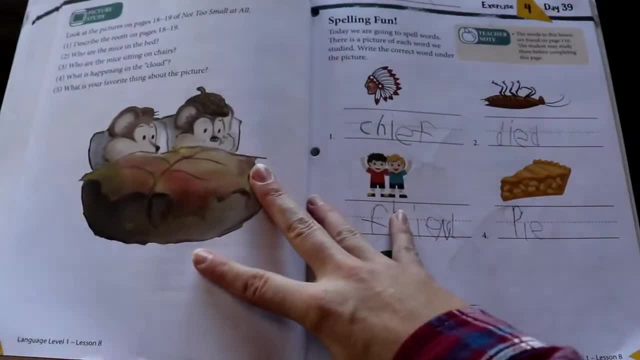 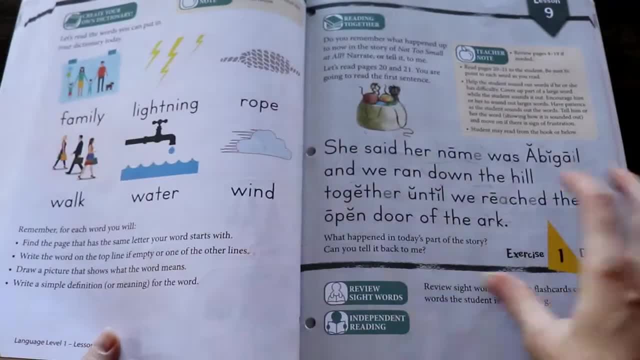 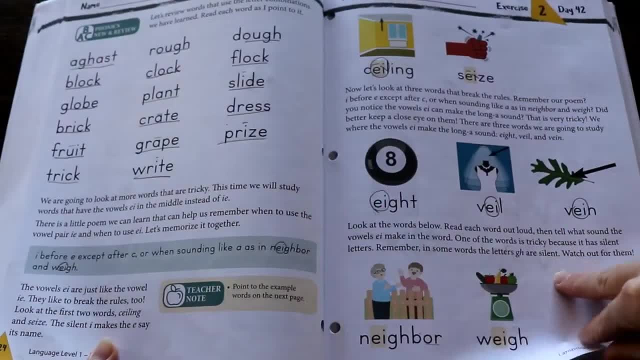 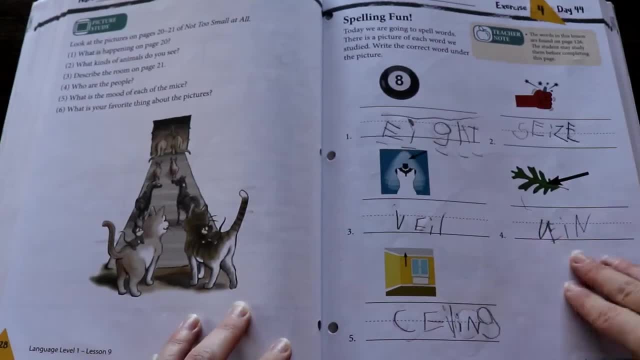 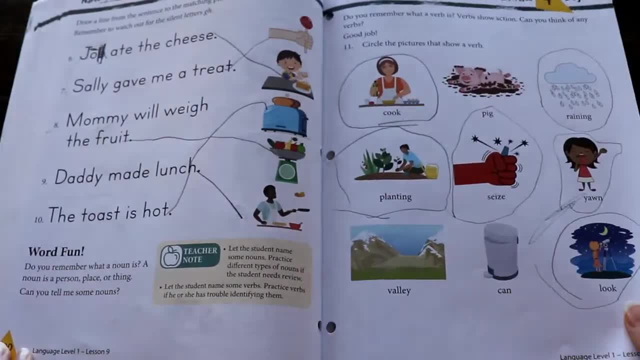 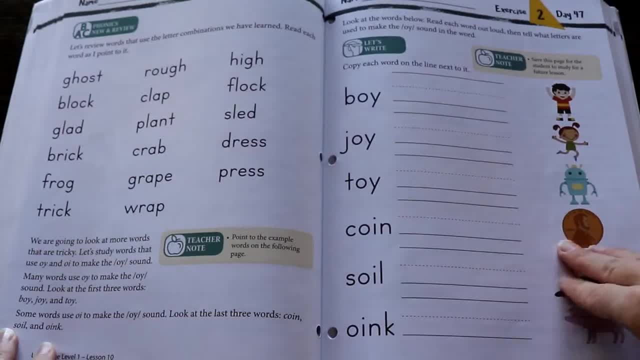 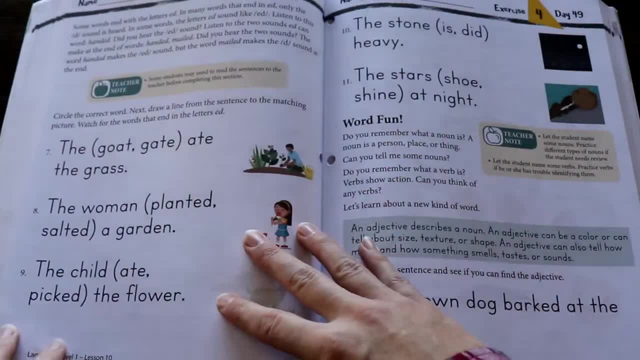 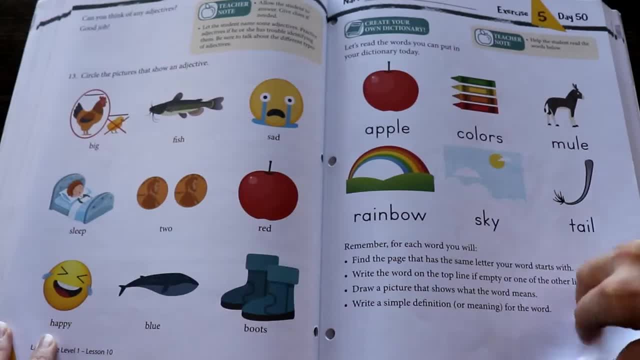 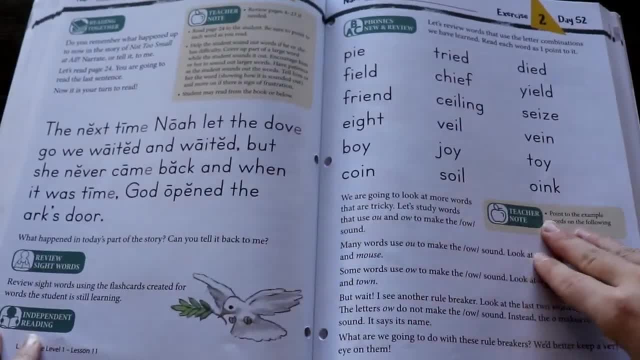 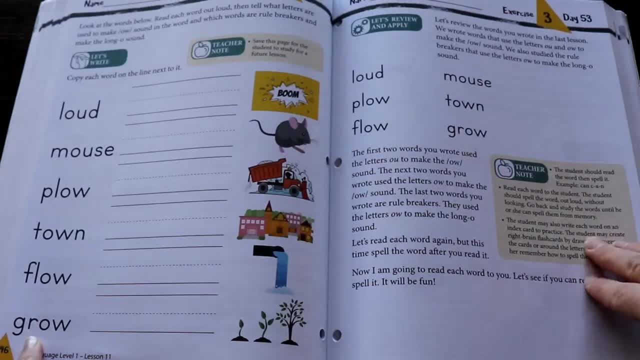 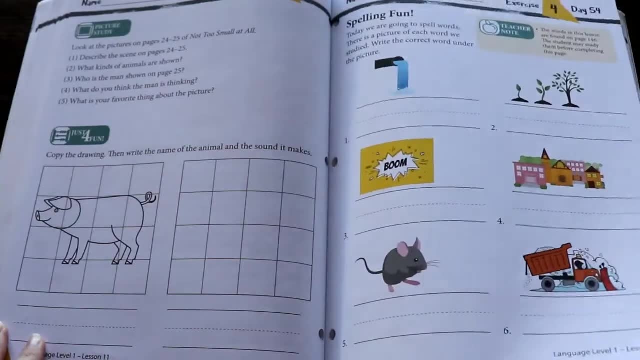 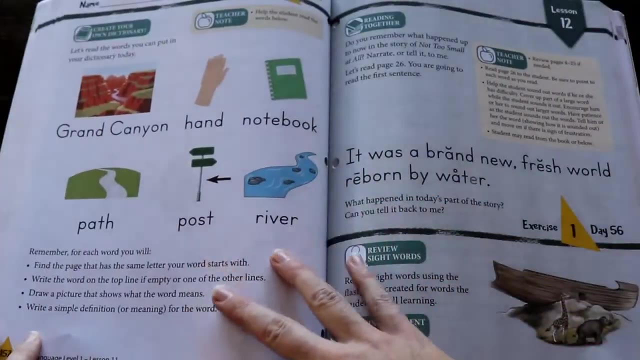 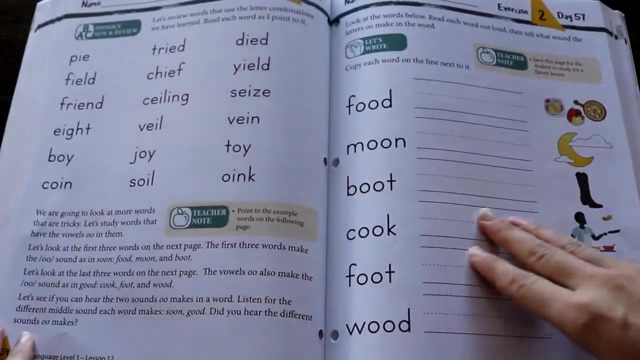 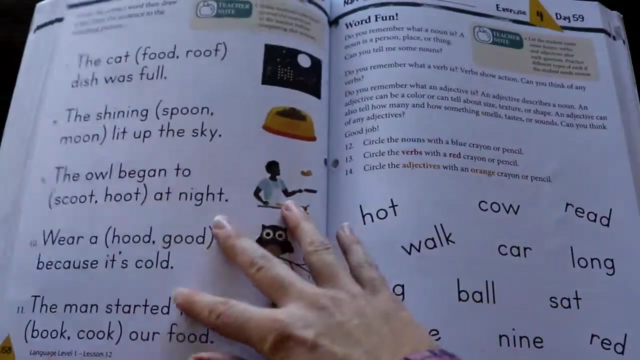 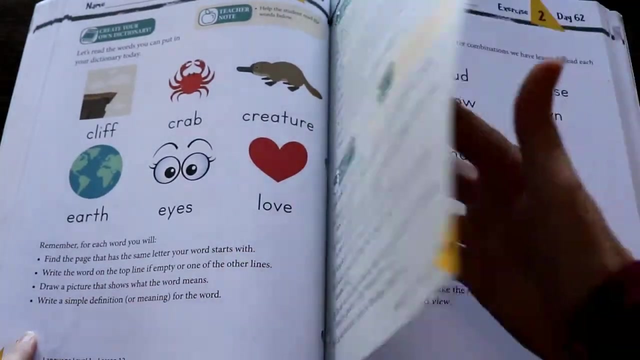 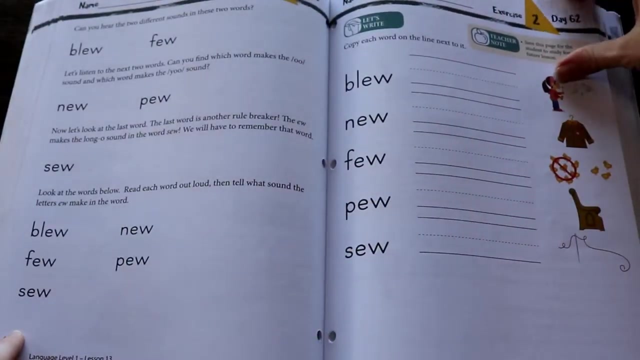 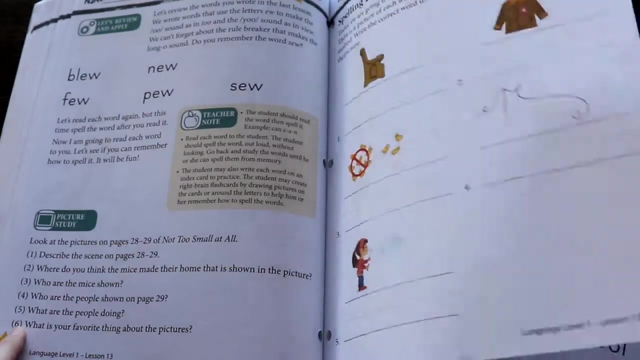 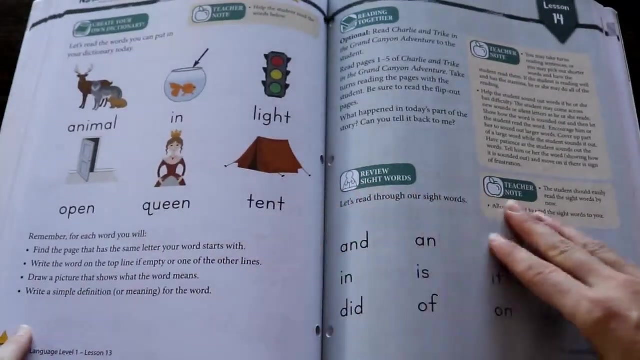 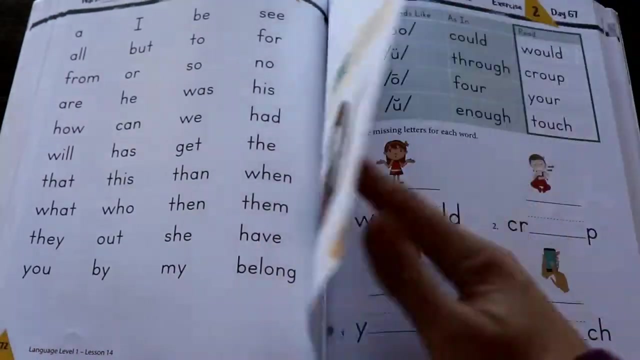 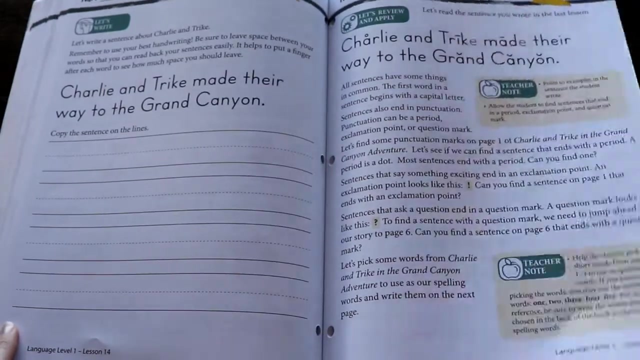 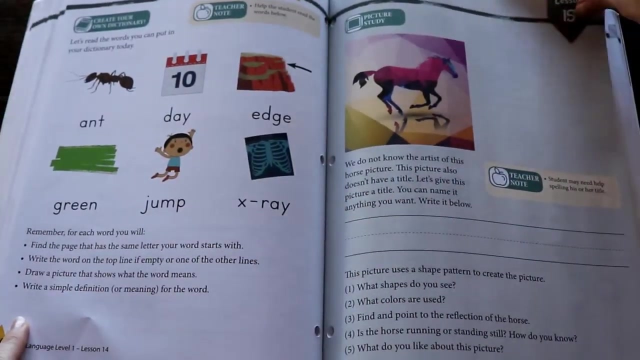 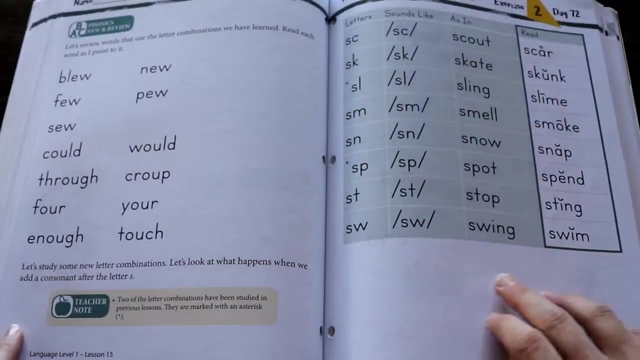 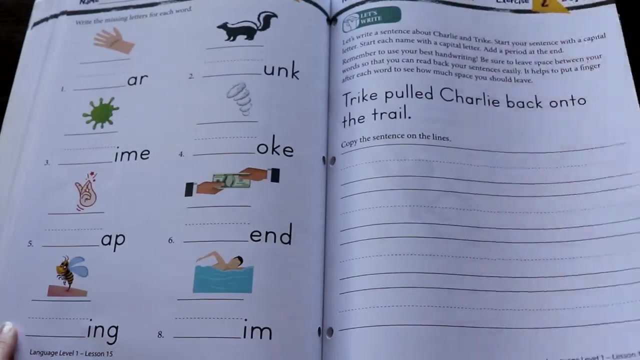